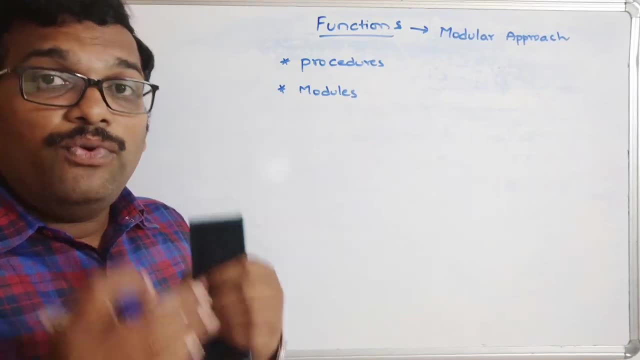 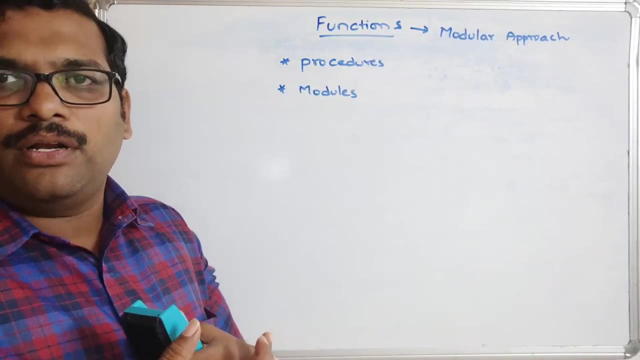 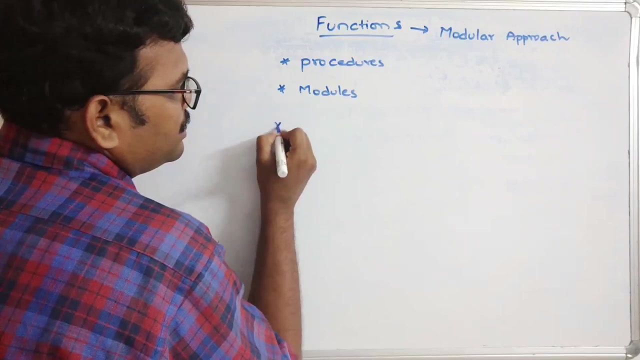 So, in order to rewrite the statements once again, we can create a small function and we can continuously. we can call that function repeatedly whenever we require. So that's why the main purpose of using this function Is code reusability- Code reusability. 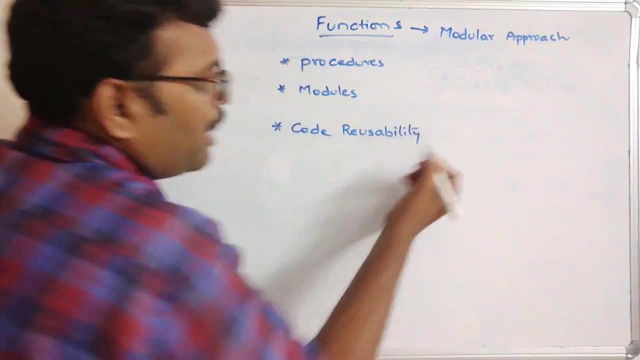 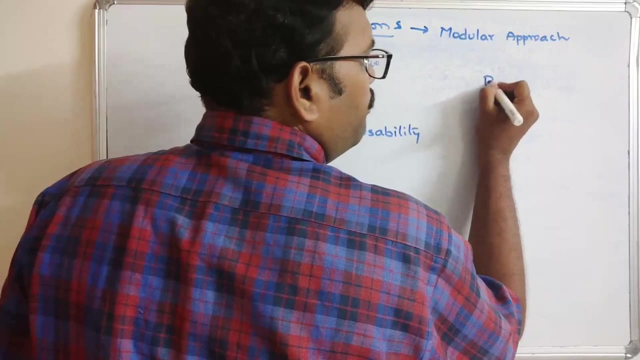 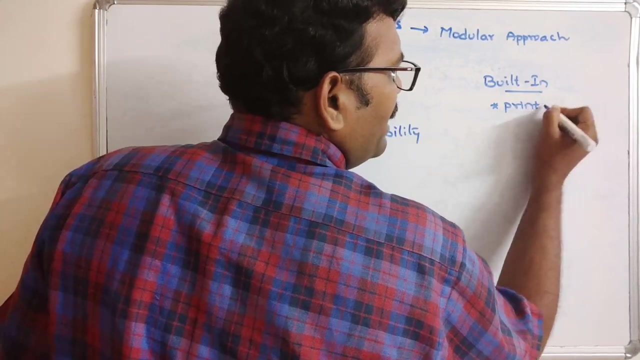 So one, only one time we will write, and multiple times we can use that particular function Example, For example. so we are having a lot of built-in functions. Built-in functions So like print function, So we are not writing any code. 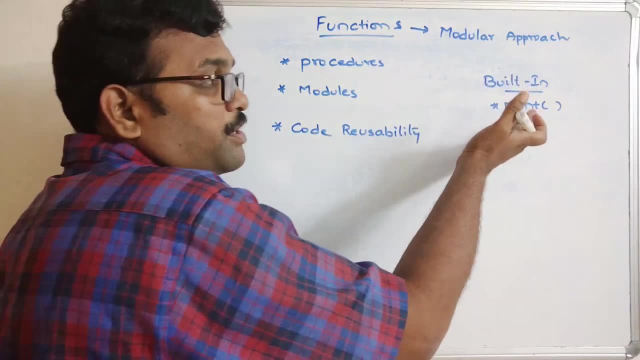 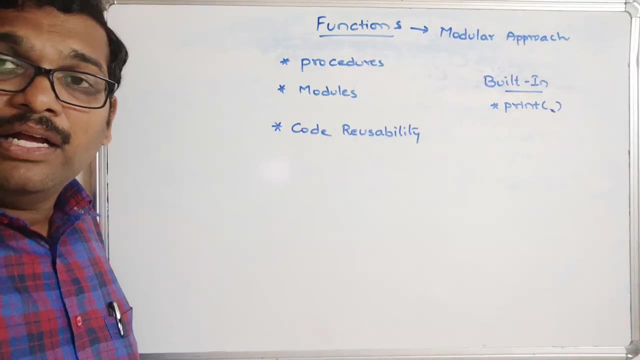 Okay, we are not writing any code, Just we are using this particular print function So that Whatever the content we are giving here, that will be printed on the output screen right. So multiple times in the same program. we are using multiple times. 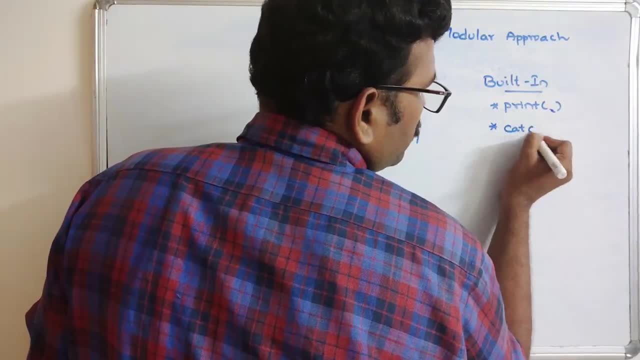 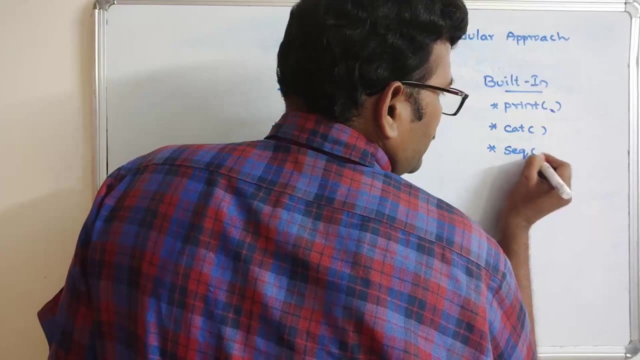 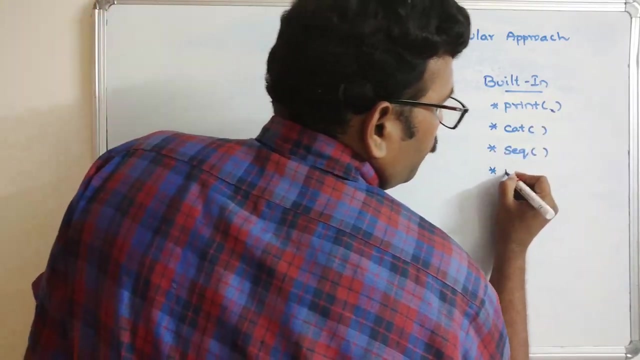 Similarly, we can use a cat function, Also, we have used this cat function. This is also an output function And similarly there are a few more functions like sequence. So, in order to find the sequence, in order to give the sequential values, we can go with the sequence in order to find the minimum or maximum. 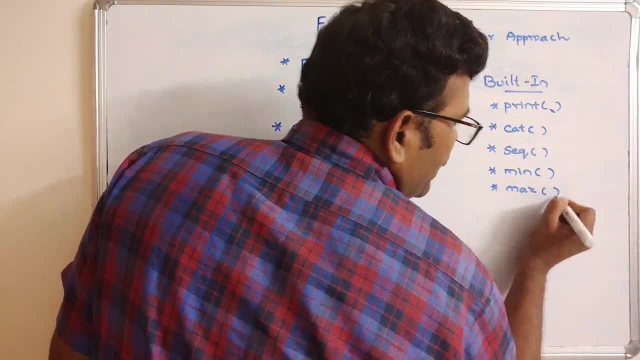 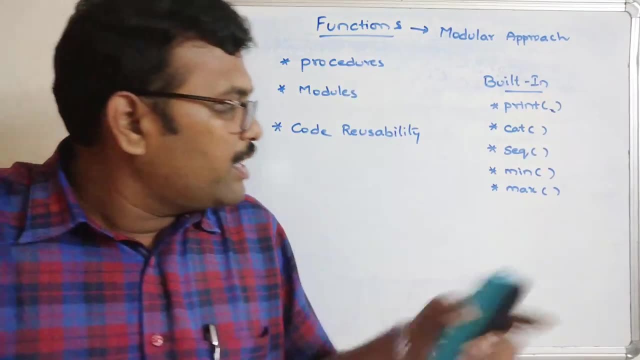 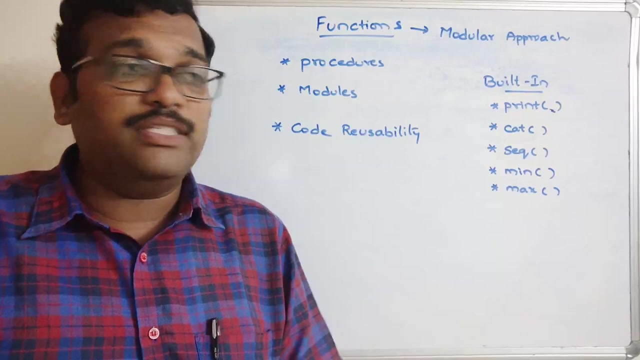 So we are having a function, We are having a function called min and max. So this will return the minimum value from the given list of elements, and it will. this max function will give the maximum value from the list of elements. So for that we are not writing any code. 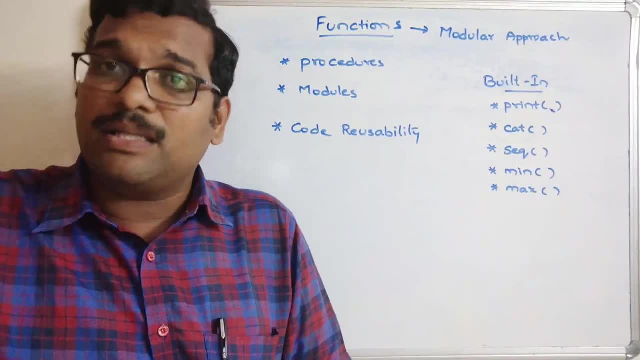 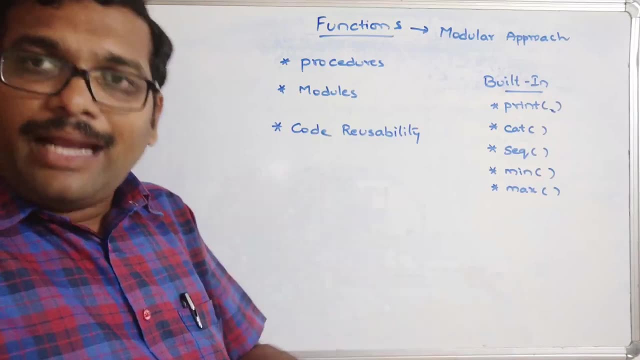 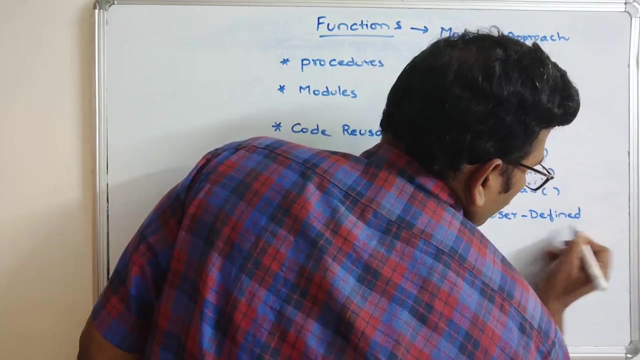 Just, we are writing this particular function and the code is available somewhere else. Okay, the code will be available in somewhere else. So, similarly, we can also write our own functions, Those we call it as a unit: User defined functions. user defined functions. 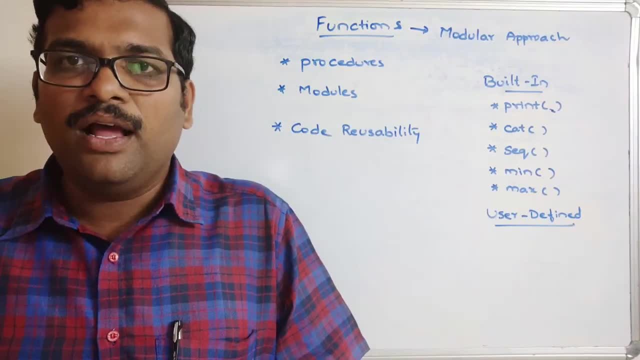 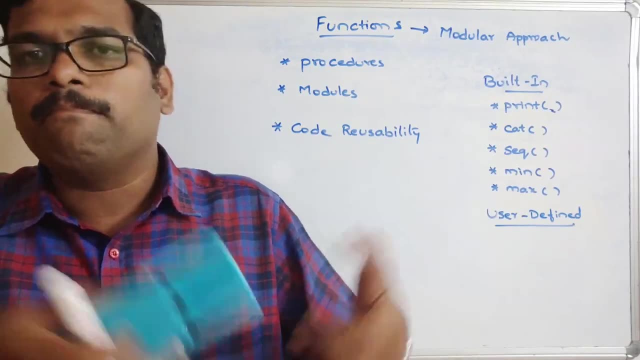 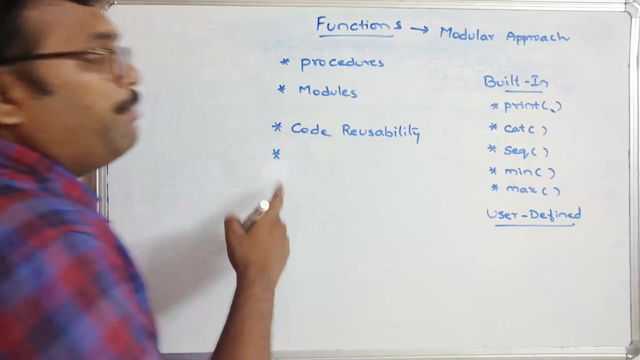 So these user defined functions were written by the user and will only once. we'll write the program and we can repeatedly call that function multiple times whenever it is required. So one is code reusability and also by going with this modular approach, Okay so complexity will be reduced. 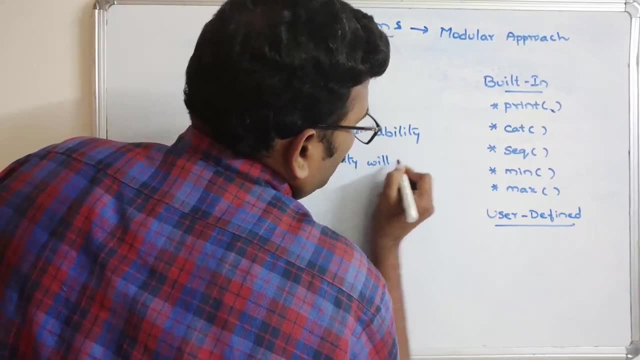 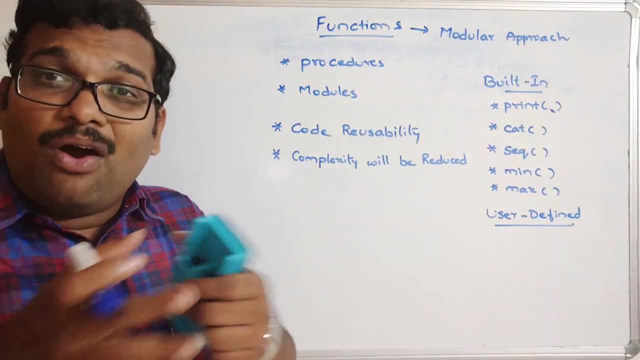 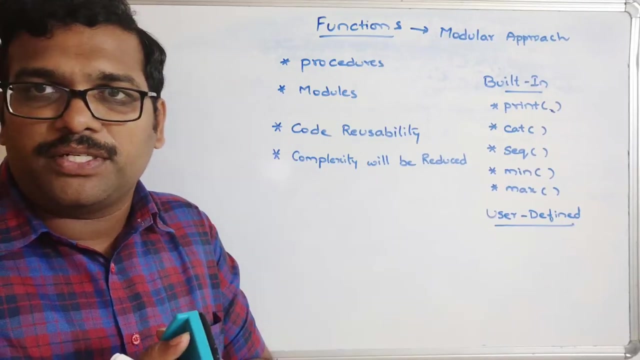 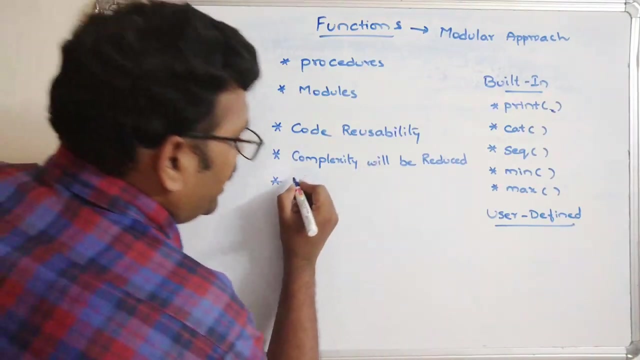 The complexity. code complexity will be reduced. Code complexity will also be reduced, So a complex problem can be divided into different modules. We call them as a functions, and later we can integrate all those functions Right So and complexity will be reduced and easy debugging. 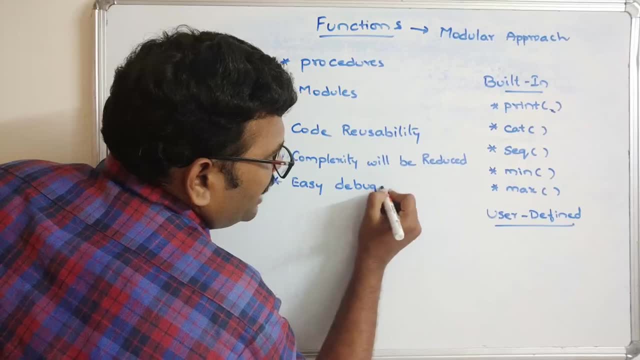 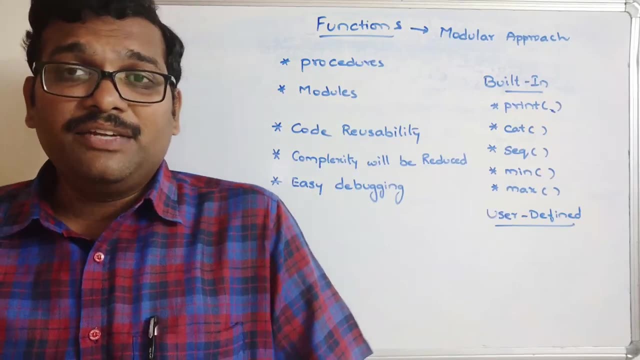 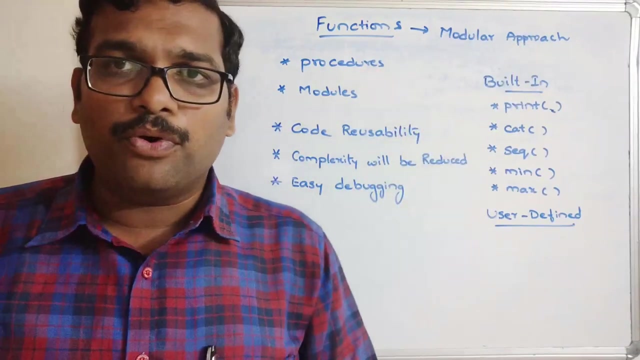 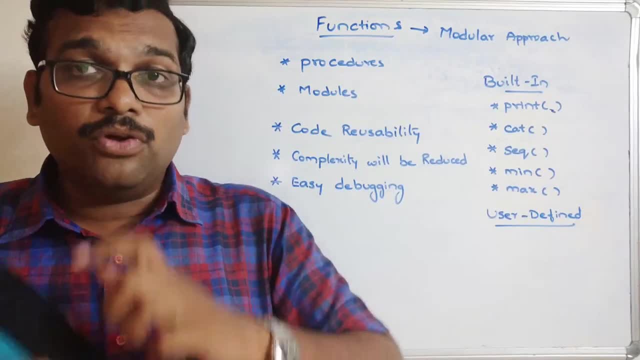 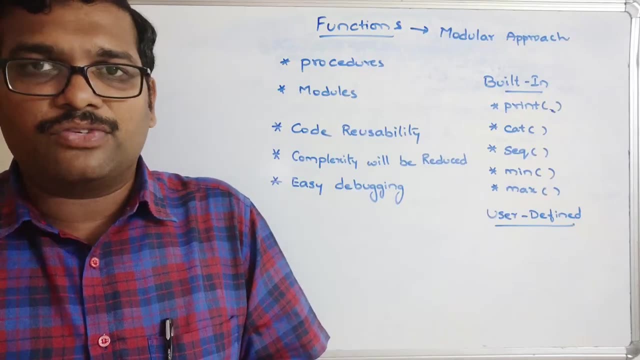 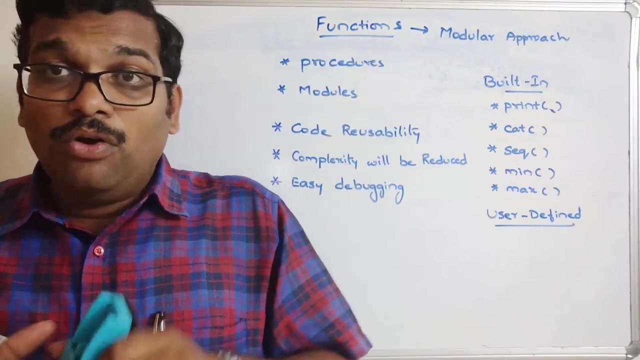 the particular module where you got the error Right. So the automatically the debugging process is easy. That means identifying the errors and rectifying those errors. We call them as a debugging, So that process will become much easier. in writing a function. So a function is also a piece of code, is also a piece of code. 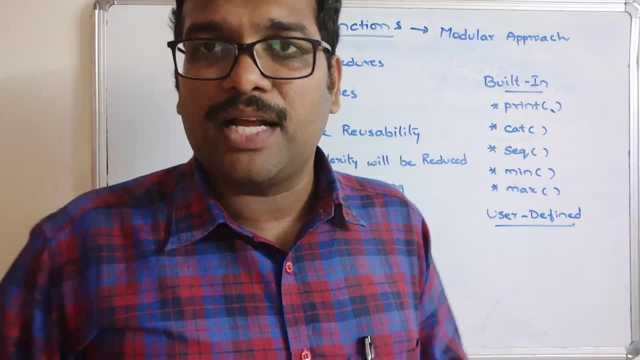 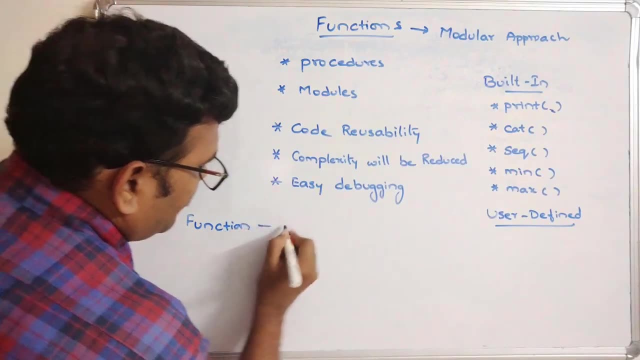 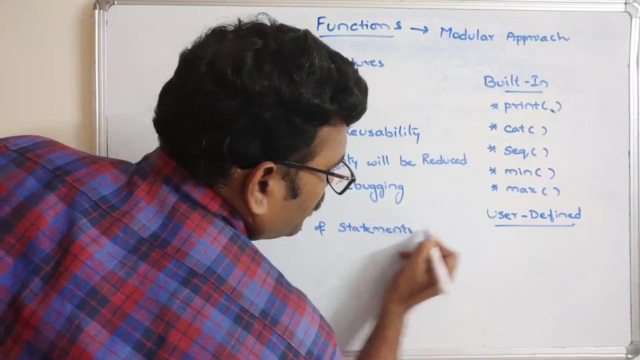 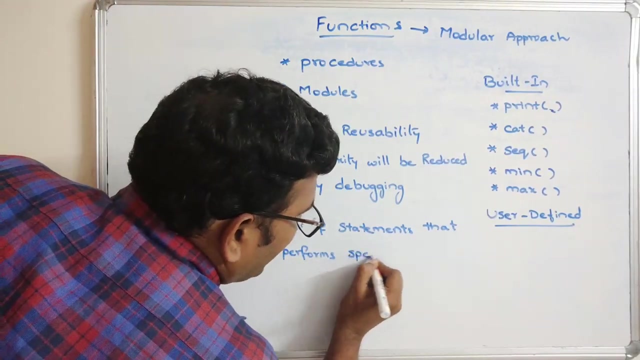 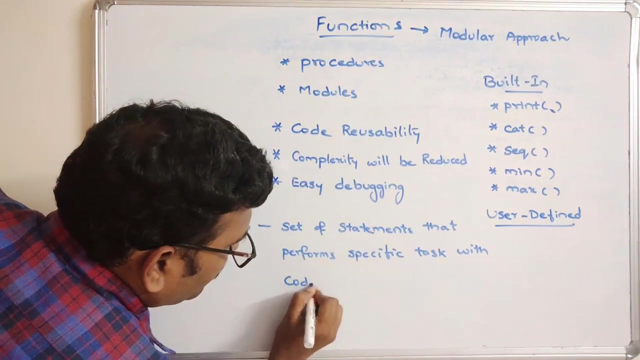 That means a set of statements that perform a specific task. Okay, Set of functions that specific task. Okay, Function. Set of statements. We can define a function as a set of statements That performs A specific task, With the code reusability. 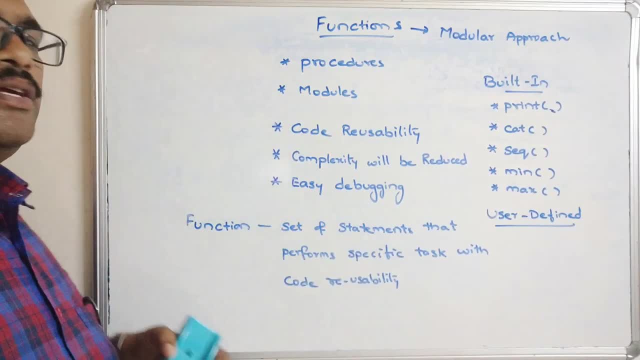 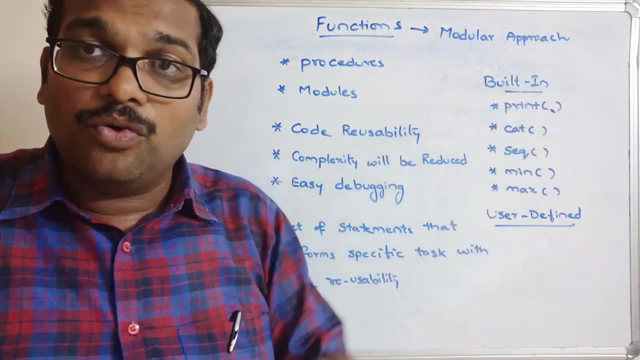 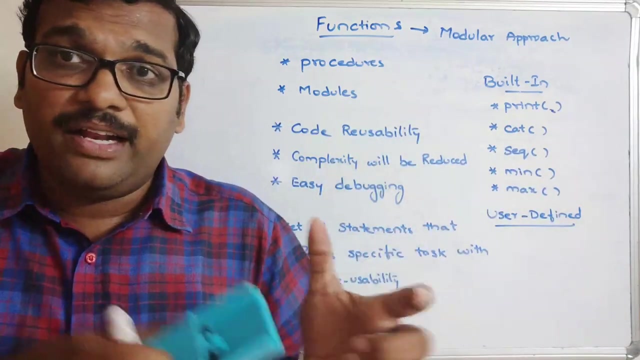 With the code reusability Right, This also function. Now there are two categories, as we discussed, built-in functions So which are already available in the R programming, So directly We can make use of those functions, You know. I mean, instead of writing the complete code, we can use these functions. 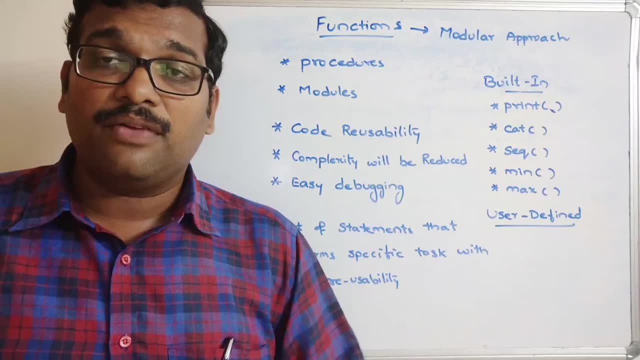 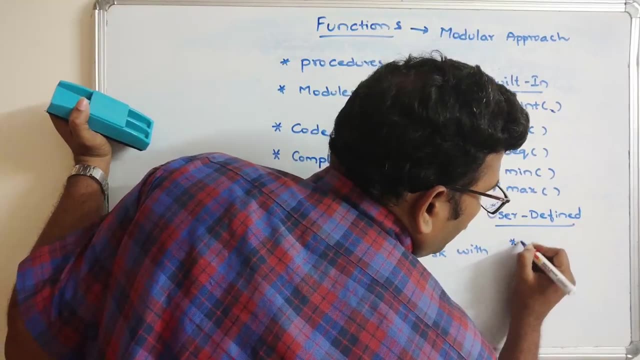 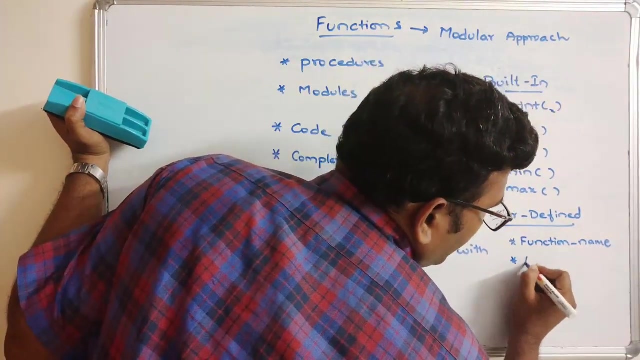 And another one is a user defined functions. So user defined functions are the functions written by the user. Okay, So, coming to the user defined functions, there will be a function name, Function name. The four things will be there- Function name. 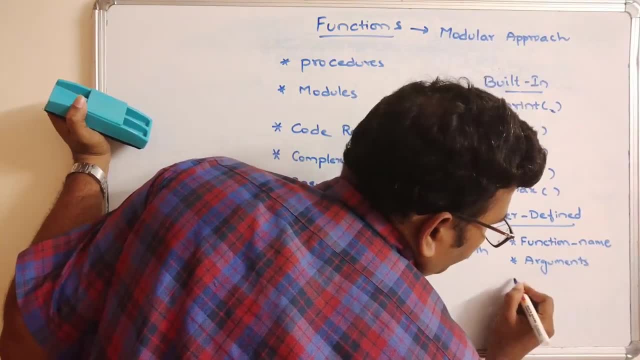 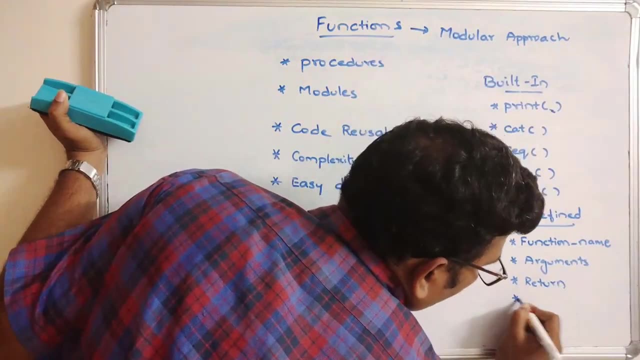 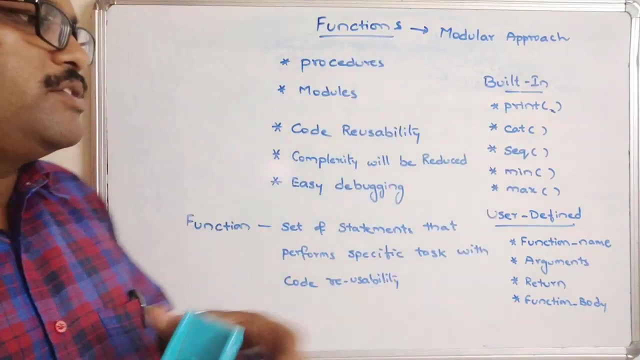 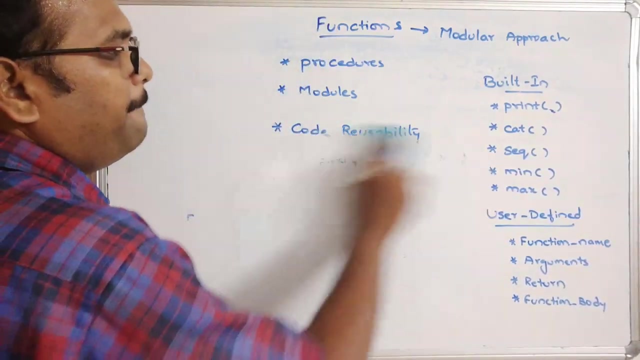 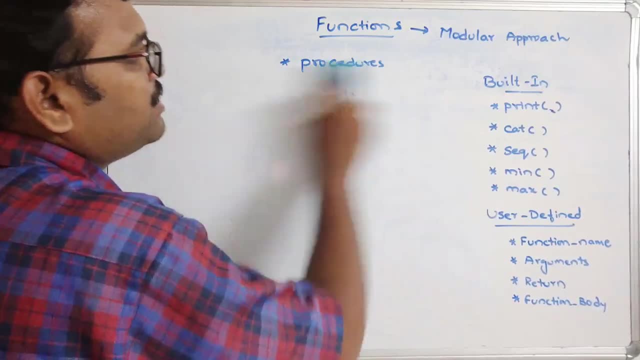 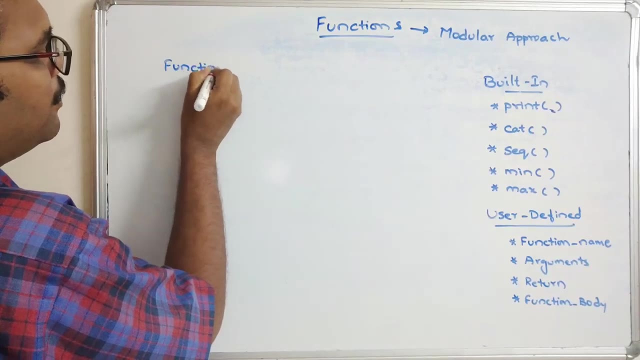 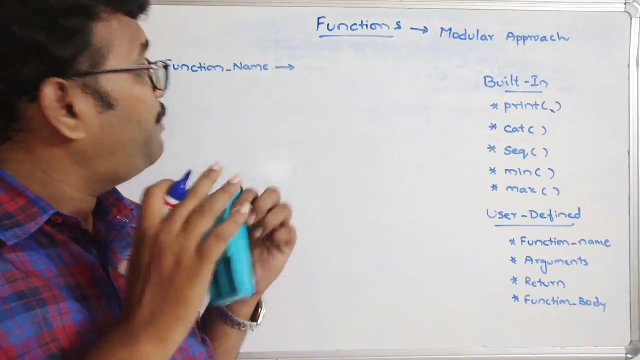 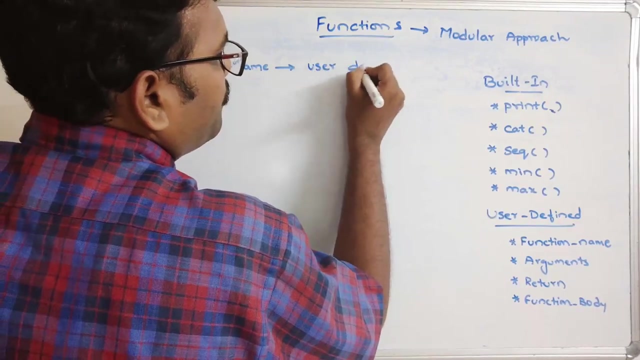 What is a function body And what is the return statement And what is an arguments Come into the function name. Is that? okay? so every user defined function will be having a user. i mean it will be having the function name which specifies the functionality. okay, so user defined name, user defined name, and we can also 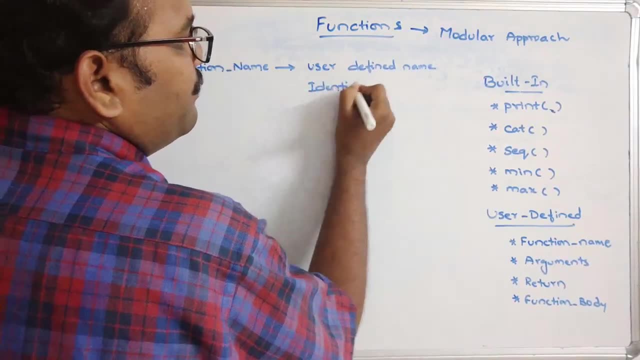 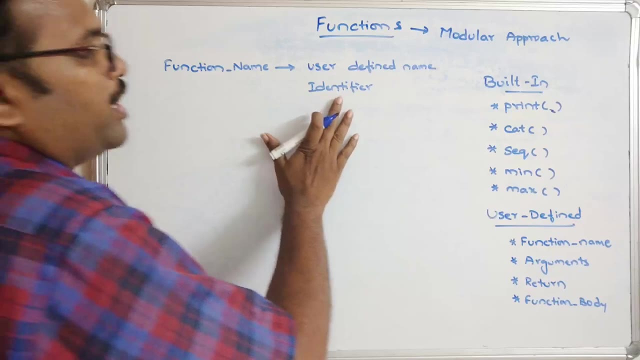 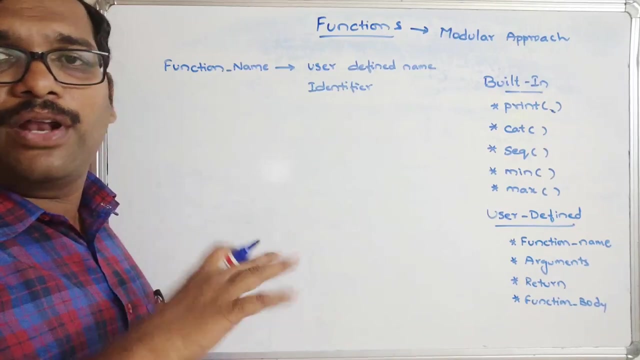 call it as a identifier. identifier, so, which identifies the memory location. okay, this is also a memory location, so which will identify the memory location? so we need to follow the rules. in our first sessions we have seen the rules should be followed by giving a name for any. 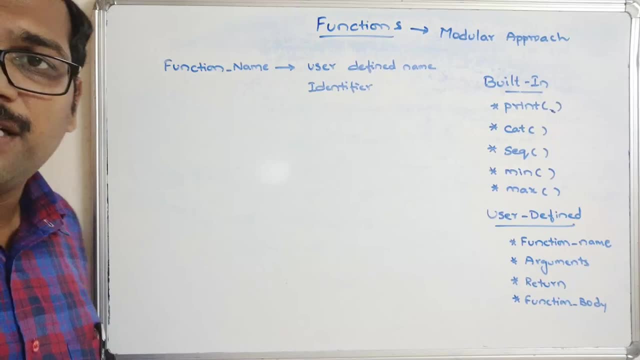 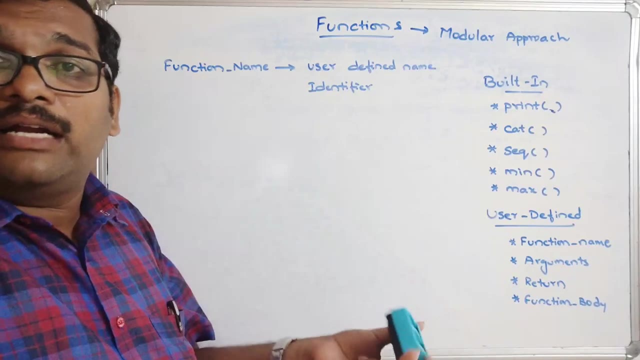 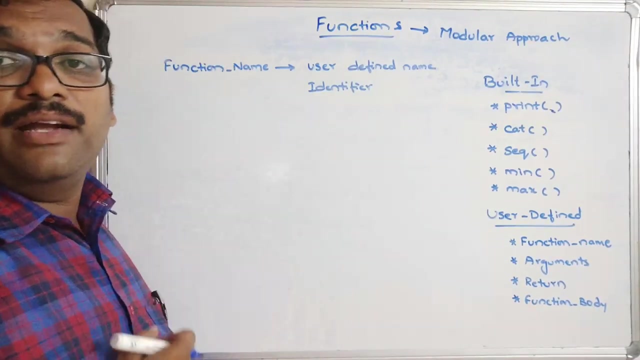 variable right, any identifier. the same thing should be happens here and we have to call that particular function with the help of this particular function name. so without giving the function name we can't access the function. so every user defined function should have the function name which gives the functionality, which shows the functionality. 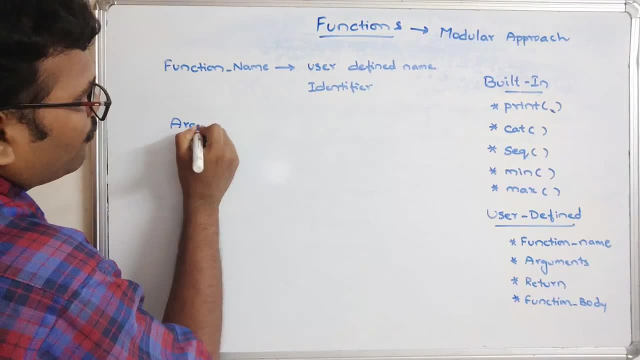 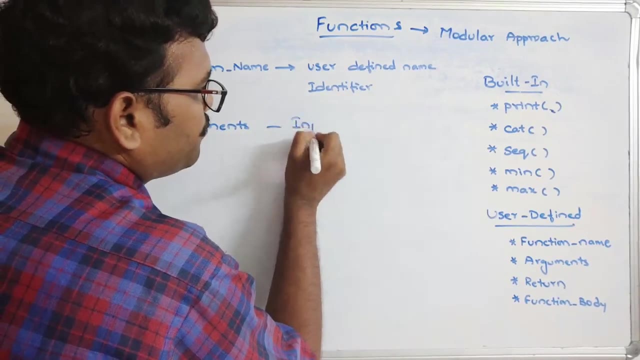 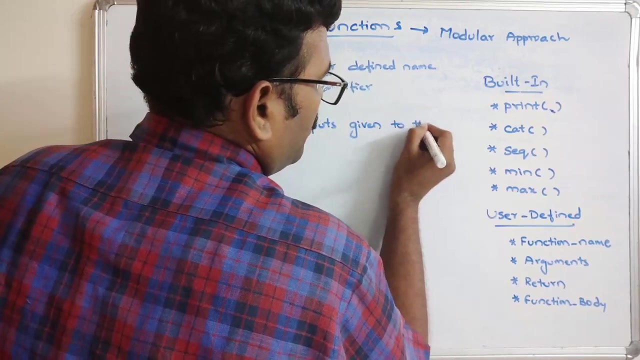 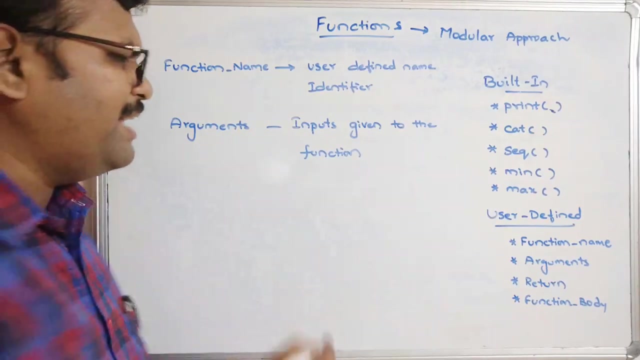 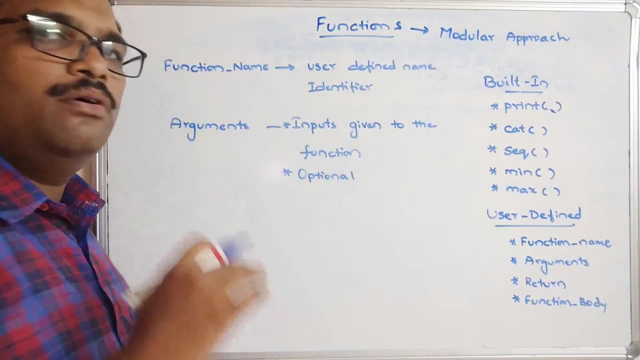 okay, and the second one: arguments. arguments are the inputs. arguments are the inputs given to the function. arguments are the inputs given to the function and these are optional. it's not necessary, it's not a mandatory to give the arguments to the function, so we can take the arguments. i mean we can take the inputs. 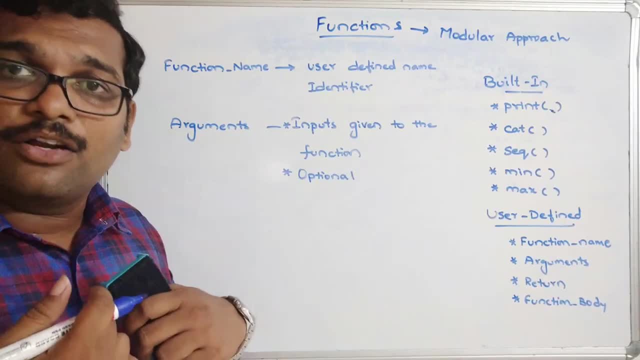 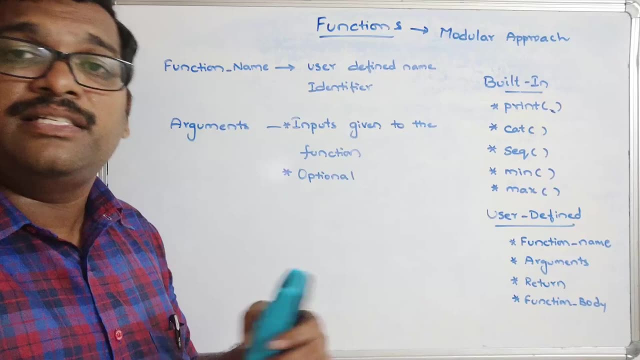 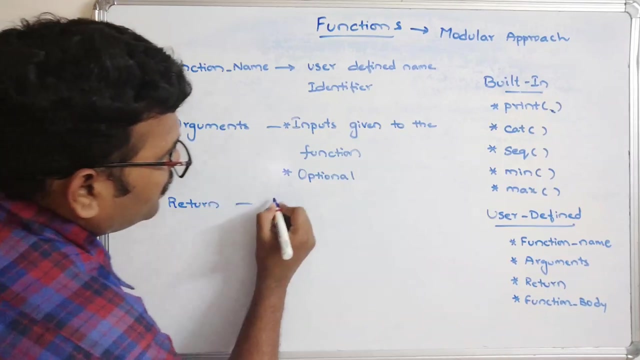 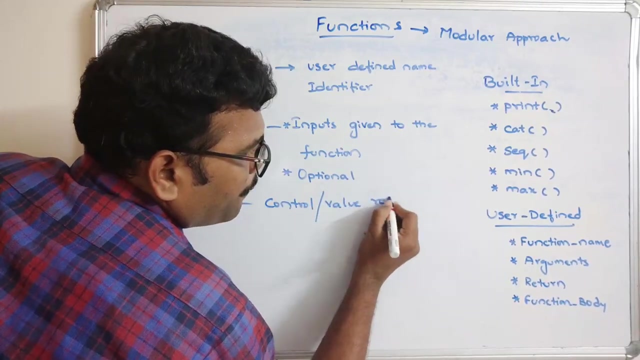 inside the function also, so we can pass the arguments or inputs from the function call to the function definition. otherwise we can take the inputs inside the function also. now the third one is a return. so this is a control or value return. control or a value return. so once the complete function user defined. 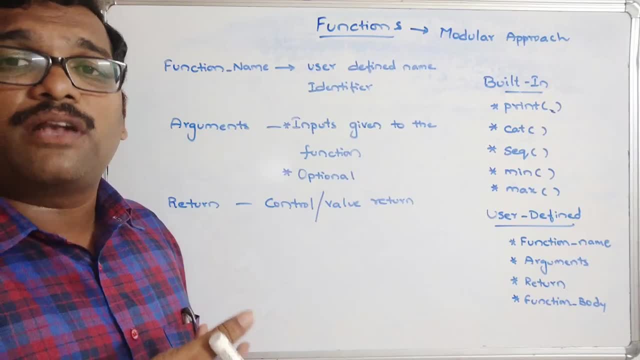 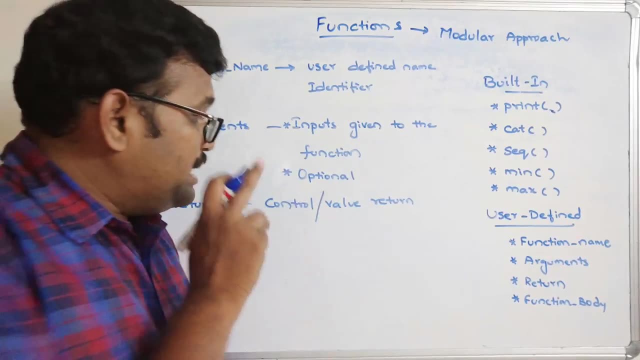 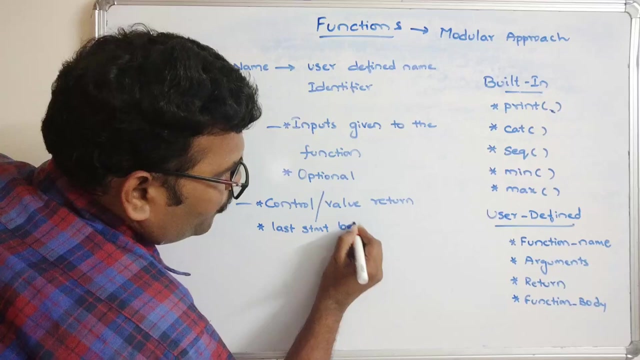 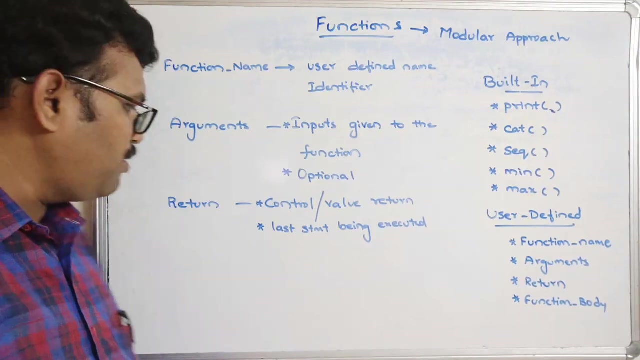 function is being executed. the result of this particular function- either it can be a value or just a control- that should be sent back to the function call. so this will be the last statement. this will be the last statement being executed inside the function. this is the last statement, okay, and the last one is. 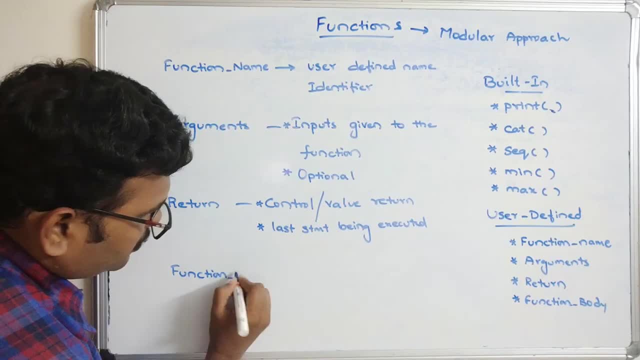 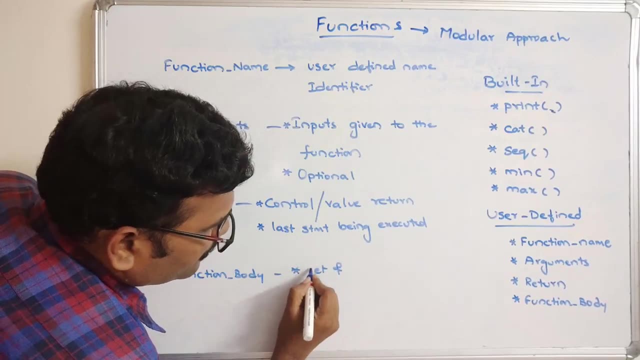 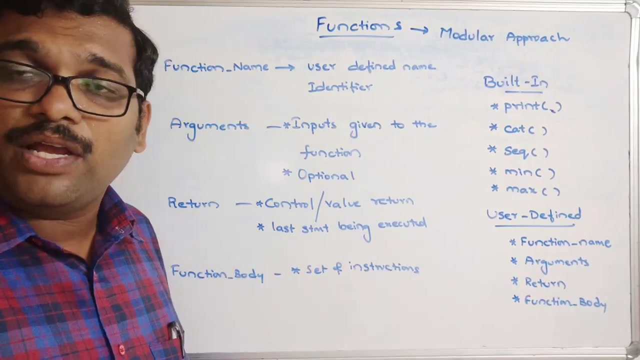 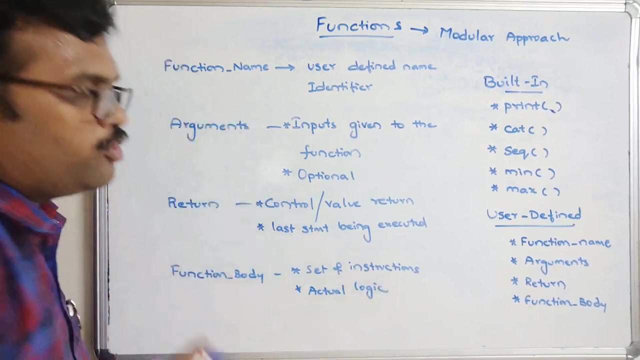 a function body. function body. so this is a place where we have to write a set of instructions. this is a place where we have to write set of instructions. okay, the actual logic. so the actual logic to be implemented, that should be written inside the function body. so if 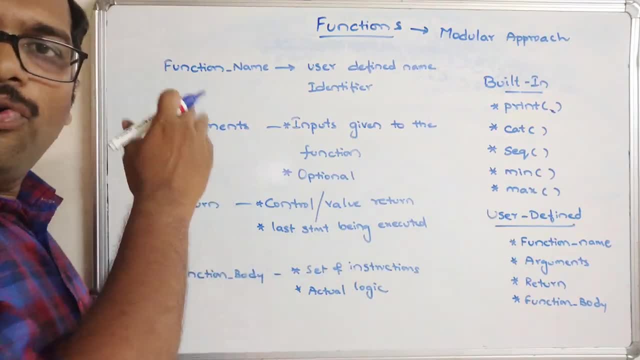 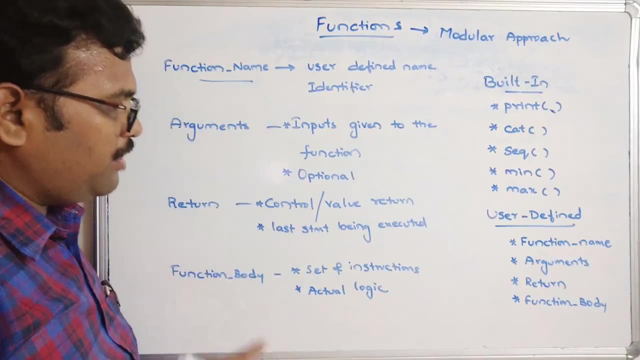 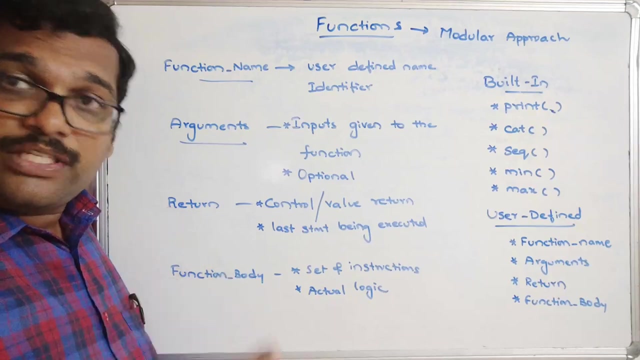 you want to write any user defined function. these four things are important, so every user defined function should have the function name and every user- I mean the user defined function- may or may not have the arguments, and the user defined function definitely will return a control or any value. 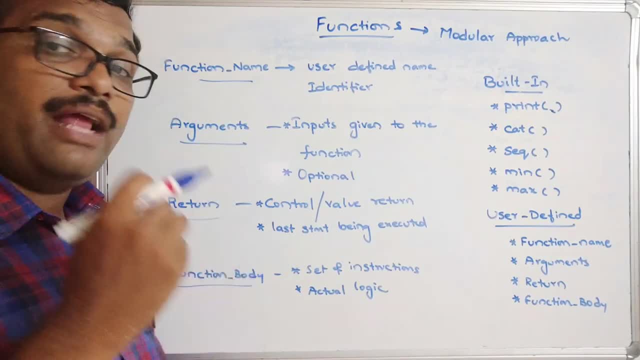 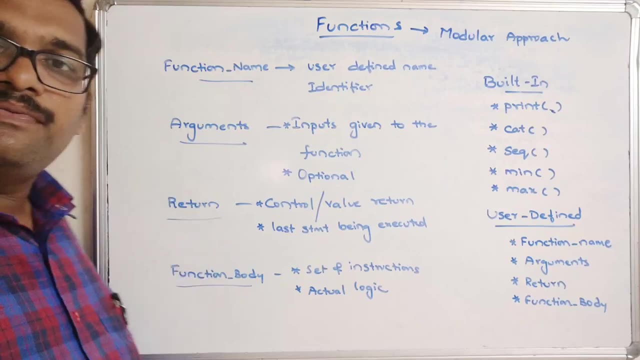 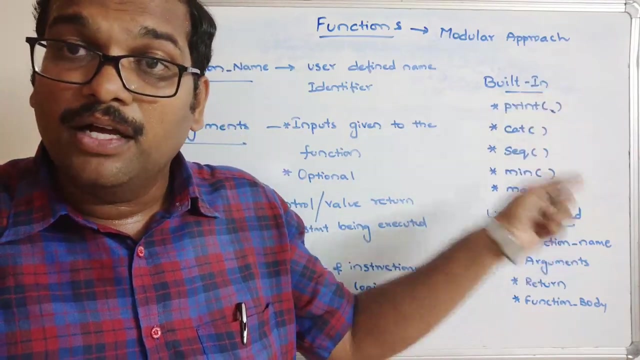 to the calling function and function body. for every user defined function, there will be some set of statements which are going to be executed should be written inside this function body. so, coming to the built-in function, just we are using these function calls, okay, so we are not writing any explicit code to. 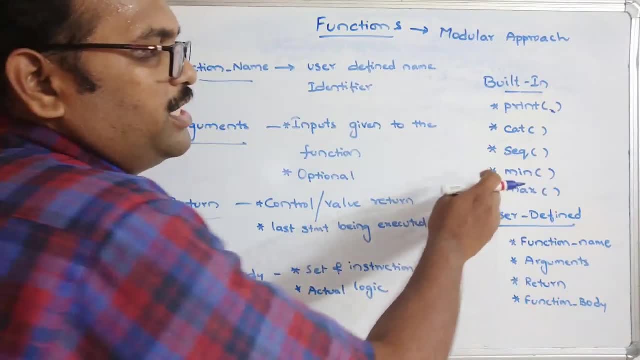 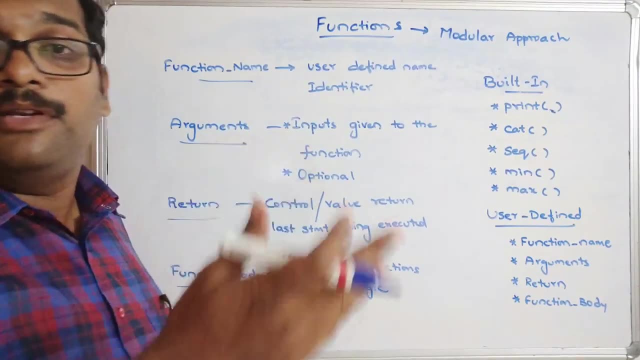 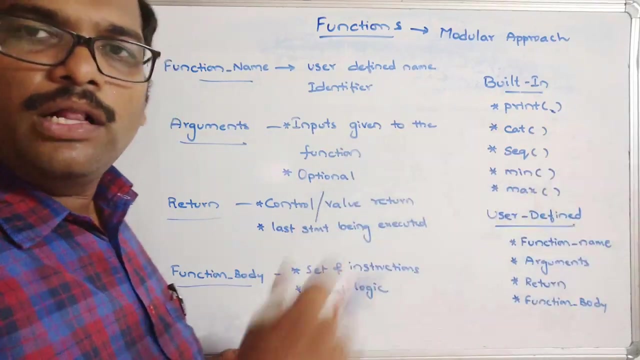 find the minimum value or maximum value. so just we are using this function automatically. we are getting the value because of the code written somewhere else. the code will be available somewhere else, and just we are calling the particular function. similarly, we have to write the code here and we can call the. 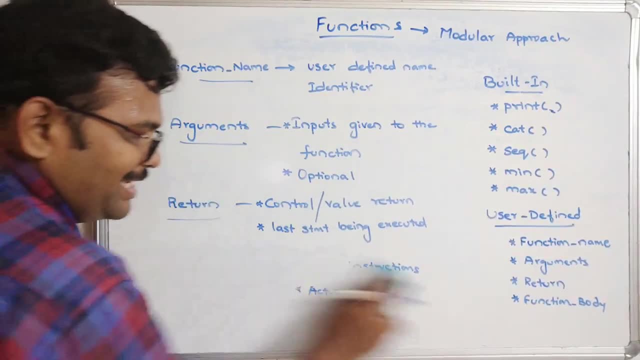 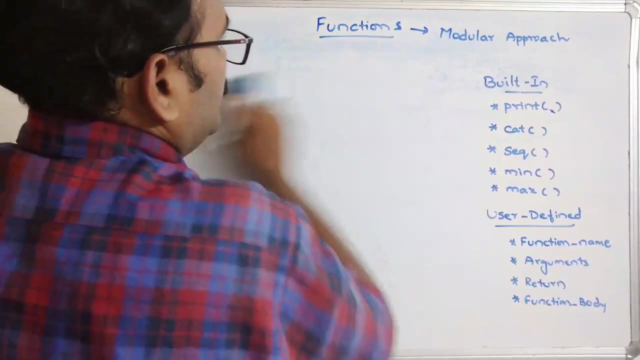 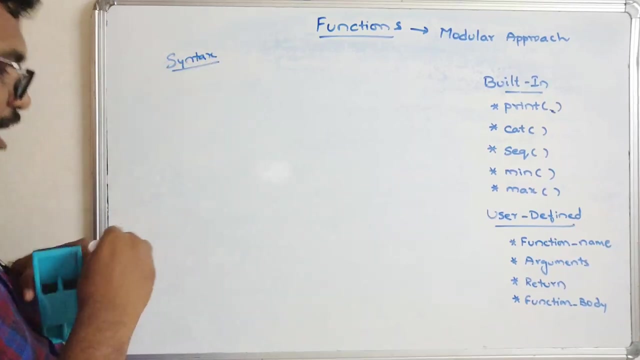 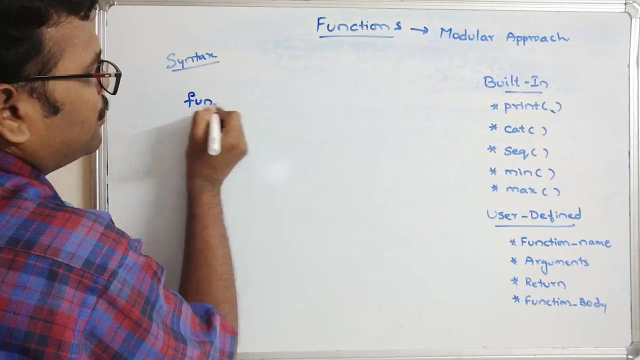 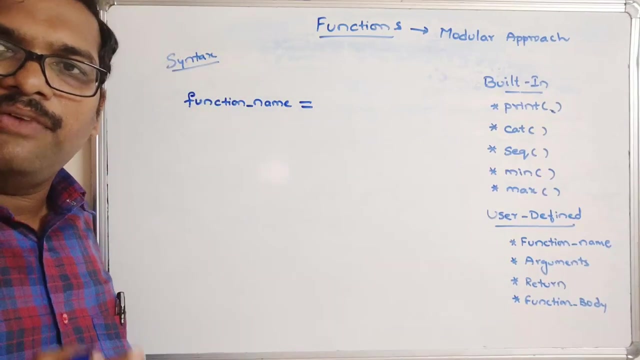 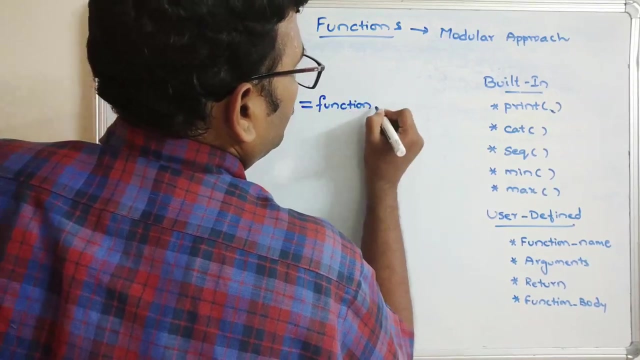 function somewhere else. okay, so let us see the syntax of this particular function, syntax of user defined function. so the first one is a function name and this is a function name is equal to every user defined function. will start with the function keyword, so function okay, and inside we can give the argument one. 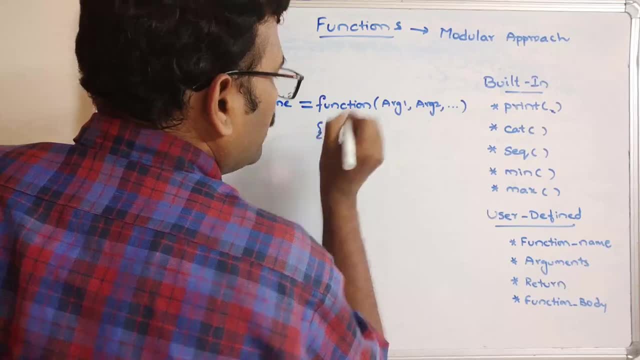 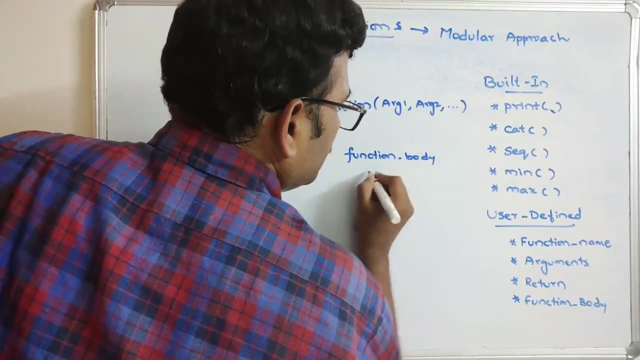 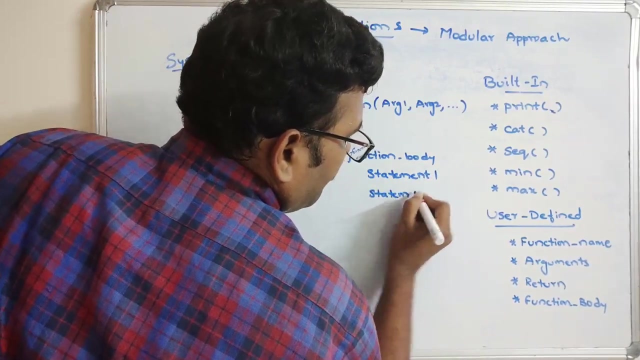 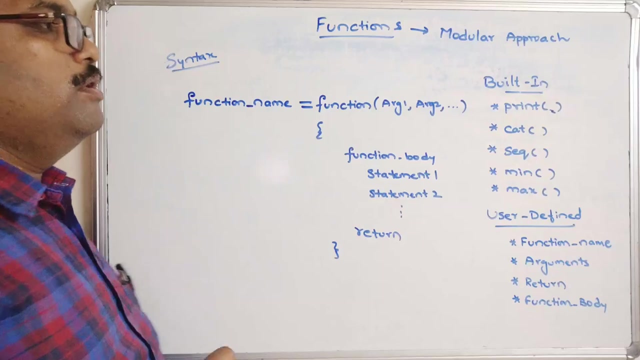 argument two and so on. and here we can write the function body. that means statements, so statement one, statement two and so on, and we can write here statement two and so on. and we can write here statement two and so on. and we can write here- this is a syntax to define a user defined function. 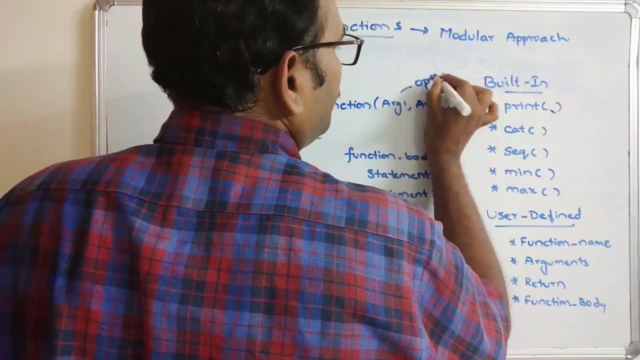 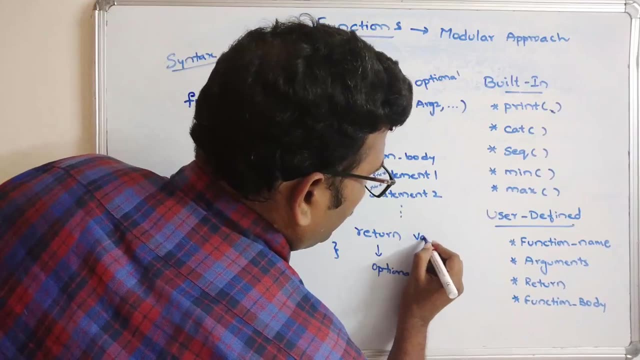 this is a syntax to define a user defined function. this is a syntax to define a user defined function. okay, and these are the optional. okay, and these are the optional and this is also optional. here you can write return value or any. here you can write return value or any. 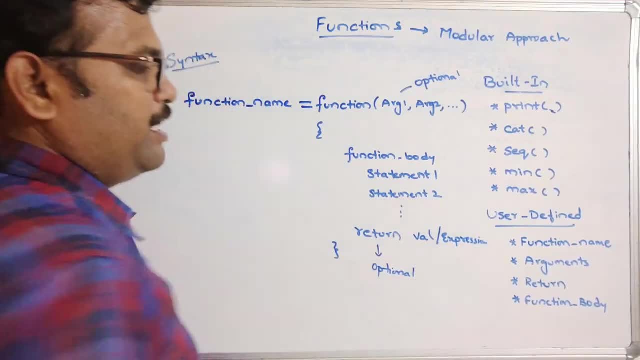 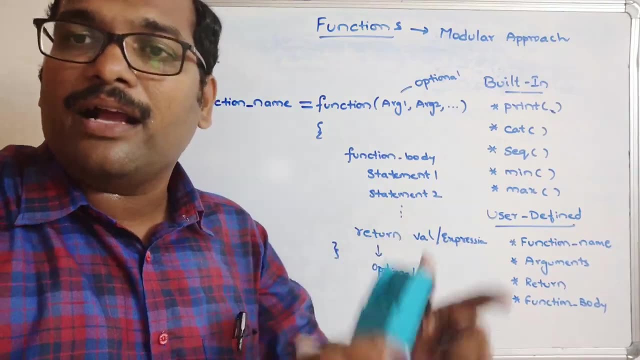 here you can write: return value or any expression. any expression return value or expression. so any expression return value or expression. so any expression return value or expression. so every function will return either value. every function will return either value or expression or a control an, or expression or a control an. 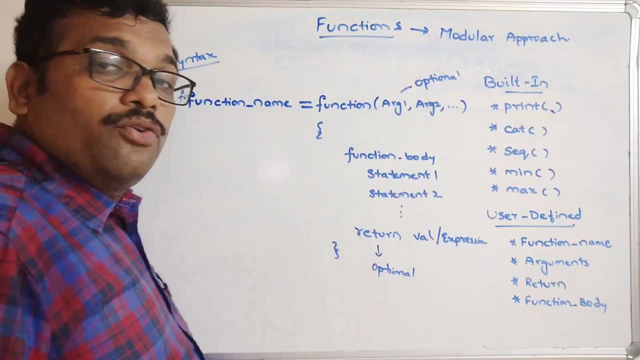 or expression or a control, an, an empty control right. so that's why we an empty control right. so that's why we an empty control right. so that's why we can go with this. it's an can go with this. it's an can go with this. it's an optional, so it's not necessary to. 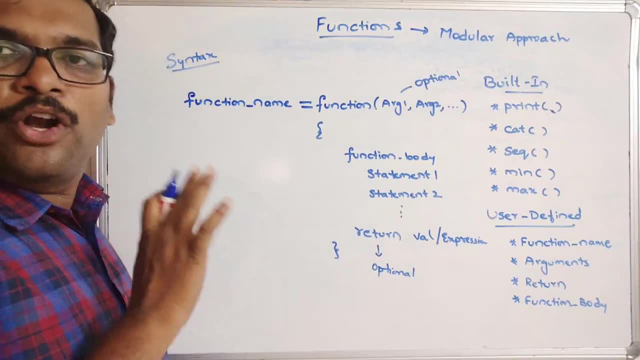 optional, so it's not necessary to optional, so it's not necessary to write down the return function. so write down the return function. so write down the return function. so we we may or may not write the written. we we may or may not write the written. we we may or may not write the written statement. 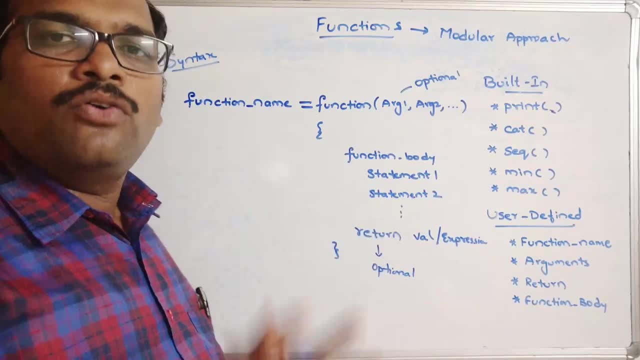 statement, statement. so if you are not giving any return, so if you are not giving any return, so if you are not giving any return, statement, statement, statement automatically. the control will go back automatically. the control will go back automatically. the control will go back to the column function. 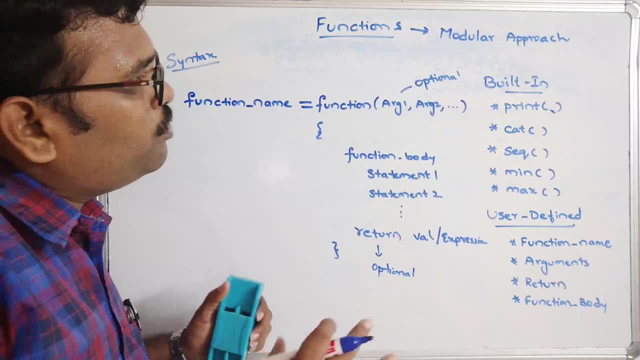 to the column function. to the column function. right. so this is the introduction, right. so this is the introduction, right. so this is the introduction to the functions concept. in our next to the functions concept, in our next to the functions concept, in our next session, we'll go in deep. 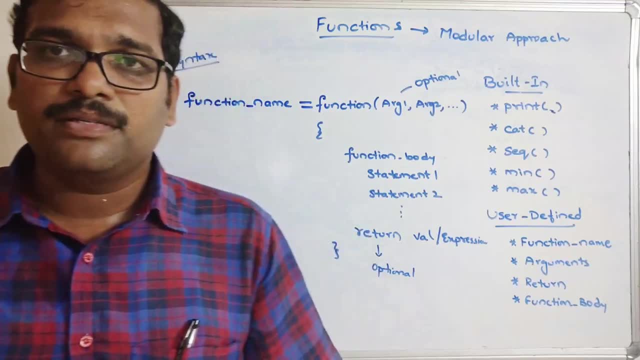 session. we'll go in deep session. we'll go in deep, in deep, and we'll see different examples in deep, and we'll see different examples in deep, and we'll see different examples. we'll execute a small programs. we'll execute a small programs. we'll execute a small programs. so demonstrating this particular simple. 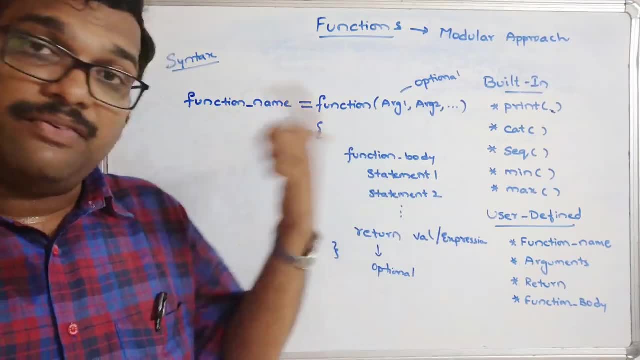 so demonstrating this particular simple. so demonstrating this particular simple: functions, with arguments and without functions, with arguments and without functions, with arguments and without arguments, and with returns and without arguments, and with returns and without arguments, and with returns and without returns. for everything we'll see, returns for everything we'll see. 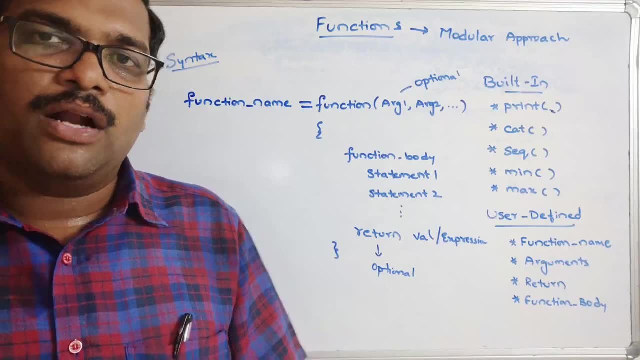 returns for everything we'll see. with an example right executing in the. with an example right executing in the. with an example right executing in the r studio. now we'll stop here. so r studio now we'll stop here. so r studio now we'll stop here. so hope you enjoyed the session and if